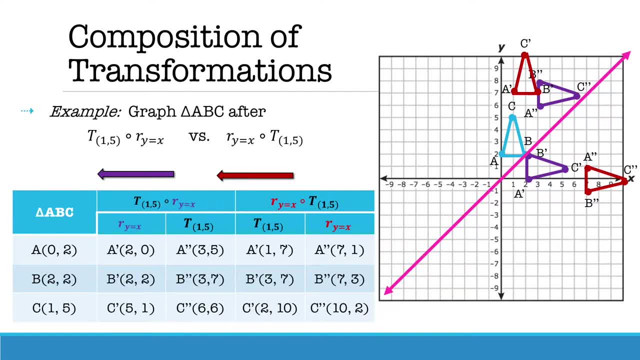 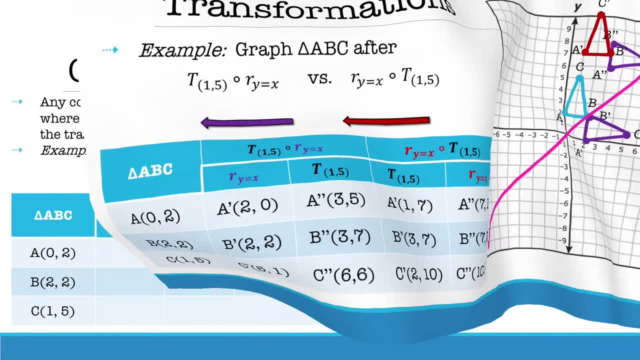 after. When comparing the two double prime images, you will see that order matters, because they do not end in the same exact position. This represents why compositions are not commutative. Let's now take a look at a special composition known as a glide reflection. 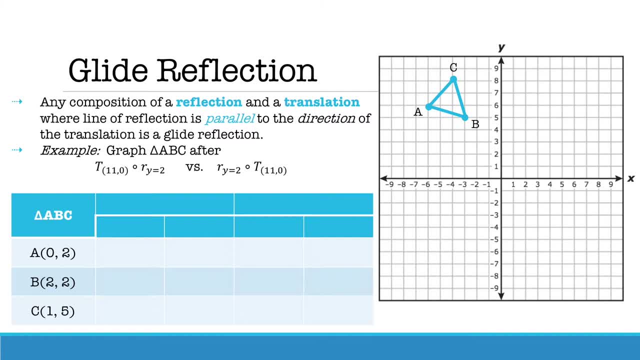 So a glide reflection is any composition of a reflection and a translation where the line of reflection is parallel to the direction of the translation. For example, here we have triangle ABC. We are going to compare it when performing a translation of: follows a reflection over the line y equals two, versus a reflection over the line y equals two. follows the translation. 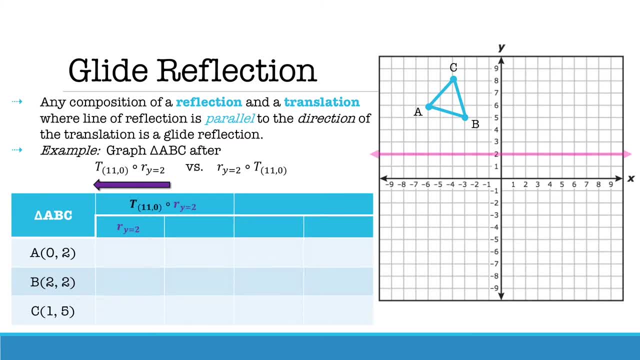 of When performing the reflection first. we are going to graph the line y equals two and reflect triangle ABC over the line, then translate eleven units to the right to get triangle ABC double prime If we were to reverse the order and perform the translation first. 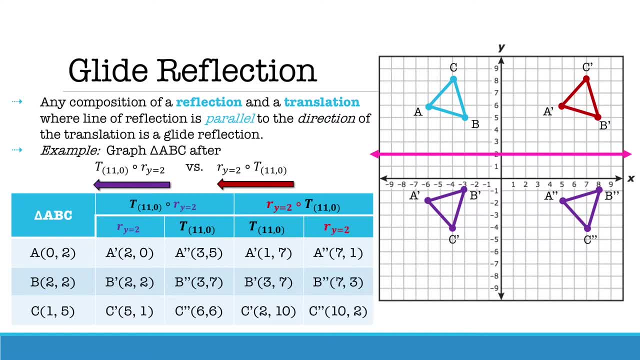 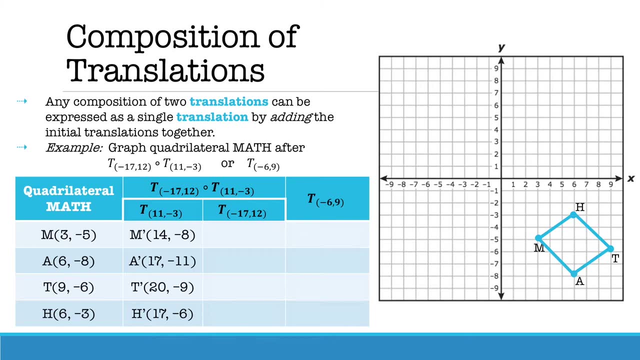 then the reflection. you will see here that your double prime image lands in this same position, therefore showing that you are doing it in the same position, which means that your drawing is now the same. showing for glide reflections. these are commutative. Let's take a look at a 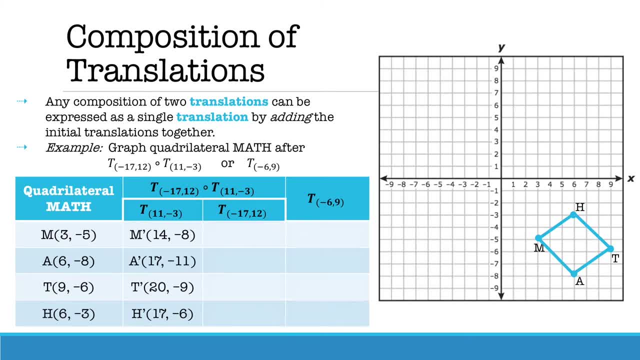 composition of translations. Here you have, any composition of two translations can be expressed as a single translation by adding the initial translations together. So if we have here graph quadrilateral math, after a translation of negative 17, comma 12, follows a translation of 11, negative 3. what we can? 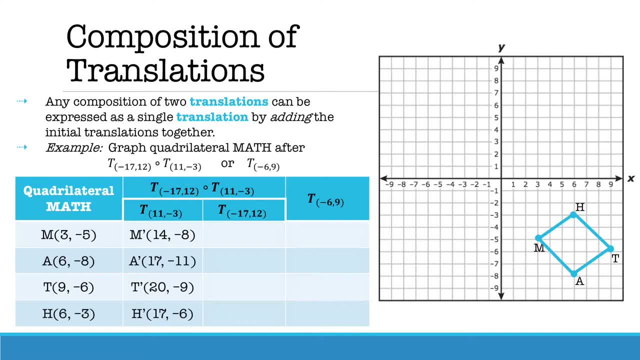 do is add the two compositions together to get a final translation of negative 6 comma 9.. So if we first perform the translation of 11 negative 3, we would get the prime image for math, then following with the translation of negative 17 comma 12 to get math double prime. 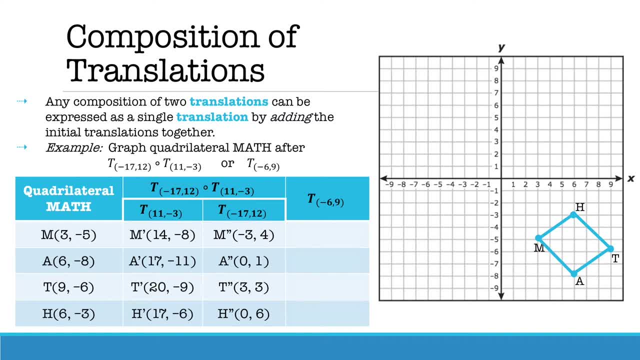 Well, 11 minus 17 would give you negative 6, and negative 3 plus 12 will give you positive 9.. So if we were to perform the single translation of moving left 6 units and up 9 units, our image will actually be the same as performing the. 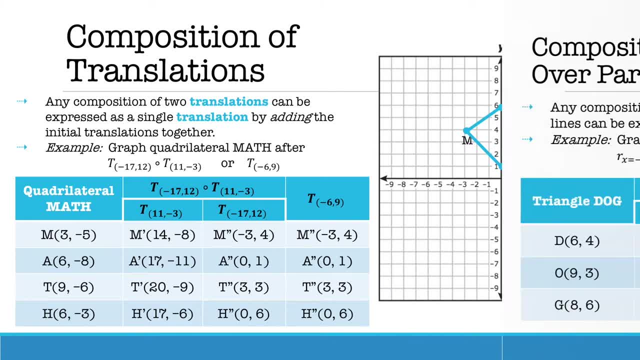 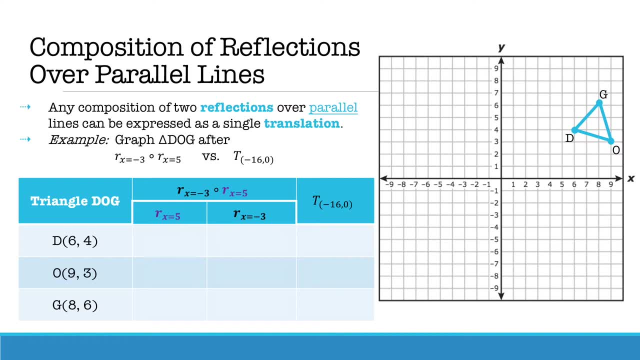 two translations separately. Let's now take a look at composition of reflections over parallel lines. Here we have: any composition of two reflections over parallel lines can be expressed as a single translation. So here we have triangle DOG. We are first going to reflect it over the line x equals to 5, then we are going to reflect it over the 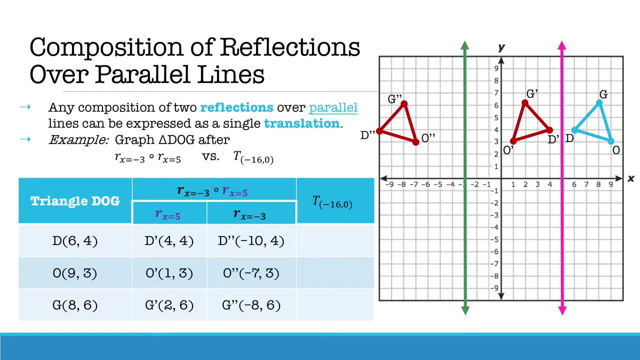 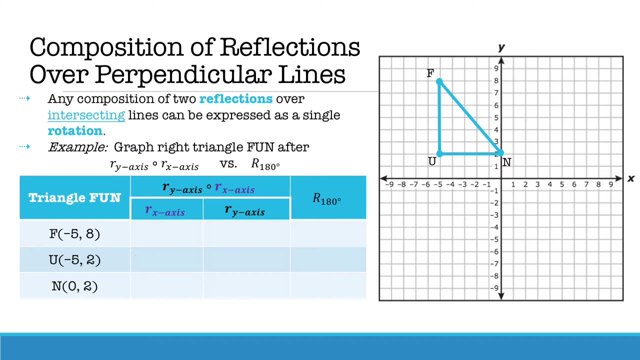 line x equals negative 3.. This is the same outcome as if we were to translate our image 16 units to the left. Any composition of two reflections over intersecting or, in this specific case, perpendicular lines can be expressed as a single rotation. So here we have a. 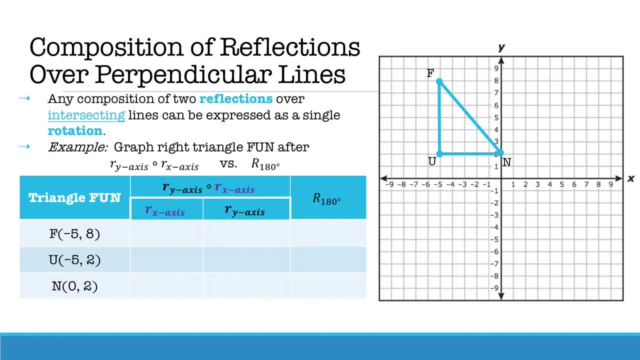 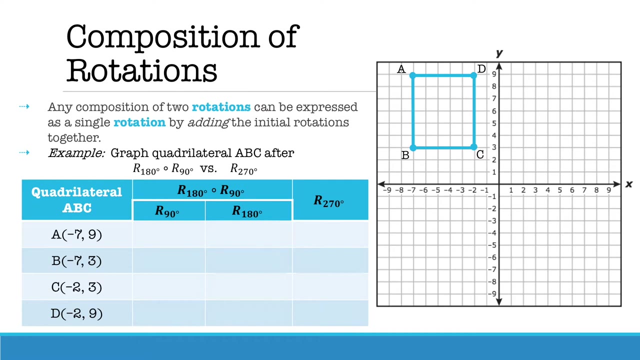 reflection over the y-axis follows a reflection over the x-axis. So if we reflect over the x-axis and then reflect over the y-axis, this is actually the same thing as rotating our image 180 degrees. Now let's take a look at a composition of rotations Similar to a composition of: 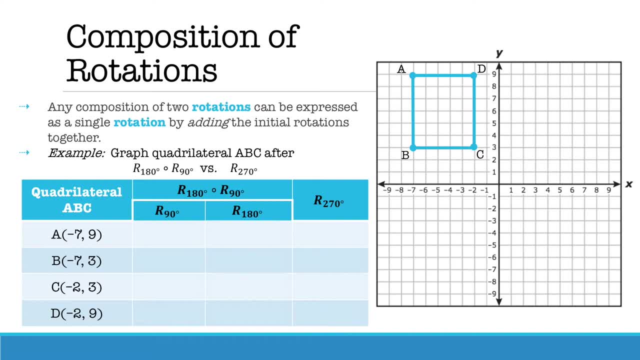 translations, where you can add the translations together. you can also add the degree measurements for your rotations to get a single rotation. So here, if we rotate the image 90 degrees counterclockwise and then rotate the image 180 degrees counterclockwise, 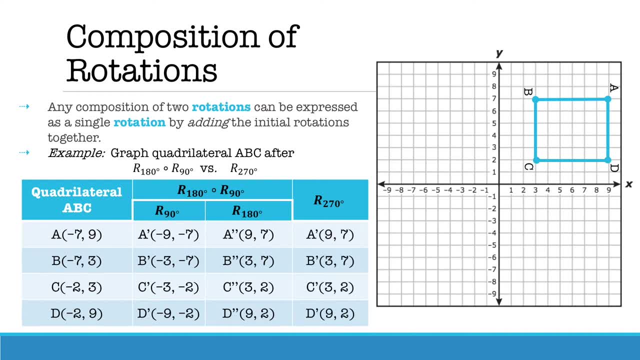 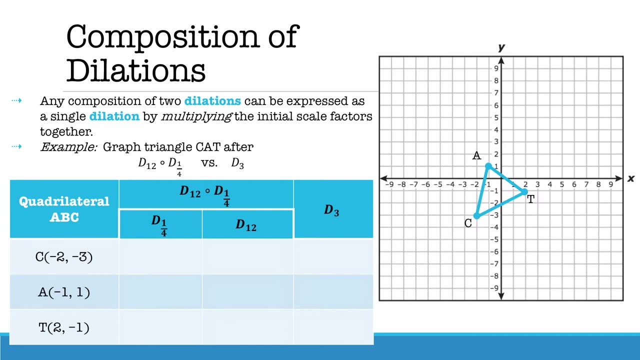 that is the same thing as rotating our image. a single rotation of 270 degrees, because 90 plus 180 will give us 270.. Let's now take a look at a composition of dilations, So similar to a composition of rotations and translations. you can combine them to give you a single.